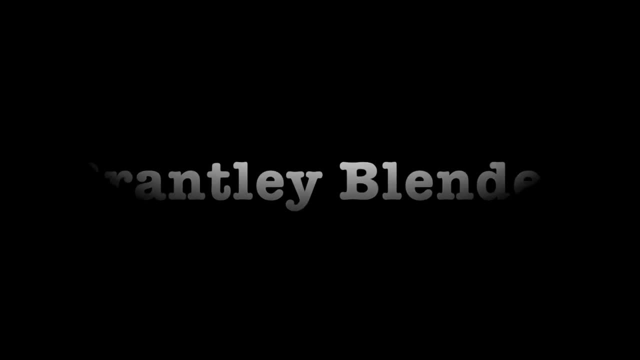 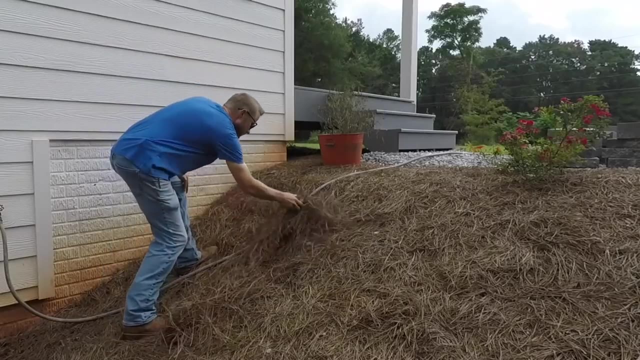 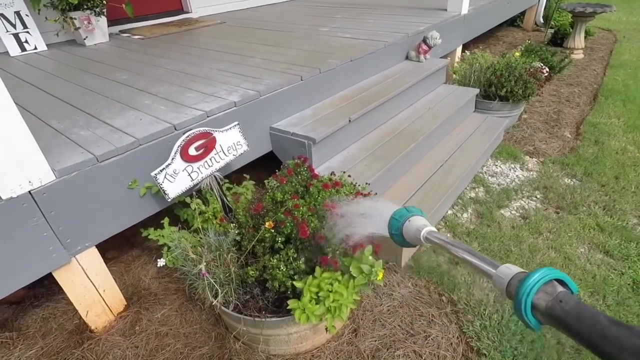 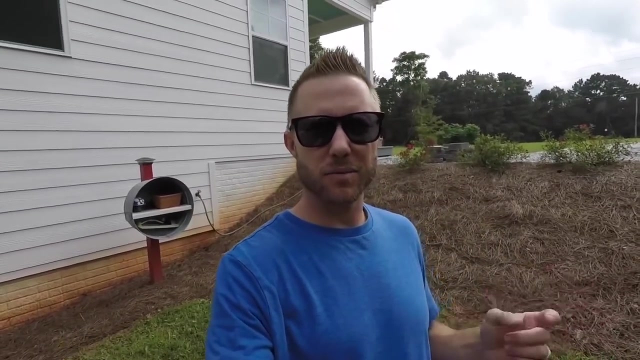 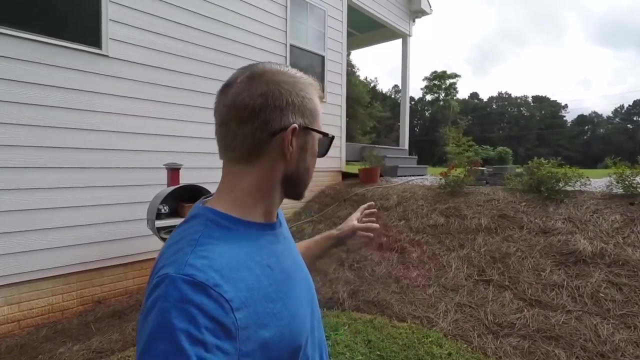 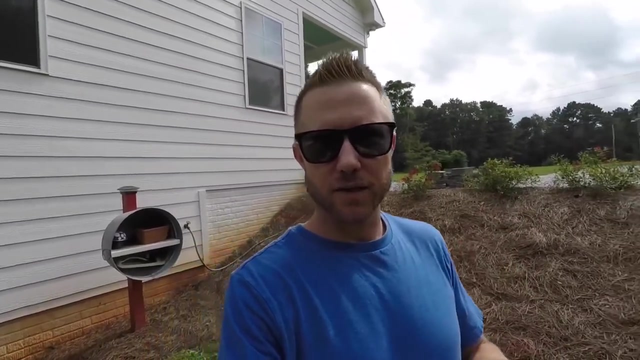 Good afternoon. It is a beautiful late September day, September 27th I think. It's like 79 degrees outside, As you can see. we need to put some stairs on this hill. I just made a video about putting pine straw on this hill and it's very slick. So today's video we're going to be building. 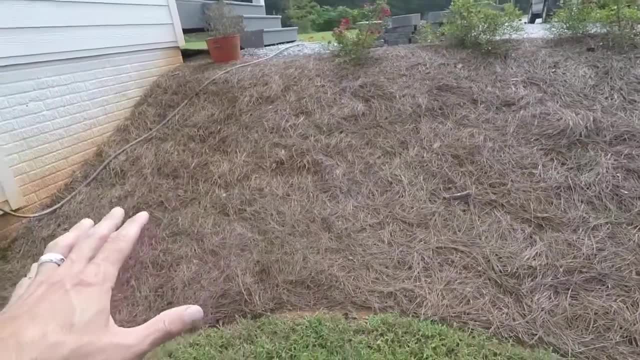 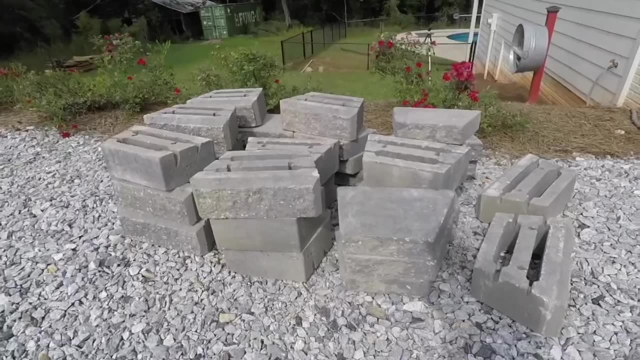 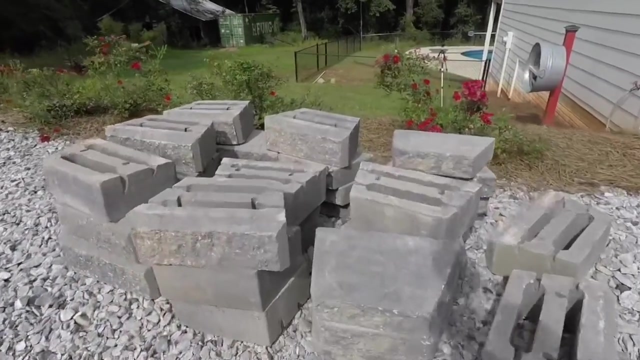 some stairs. We don't have an exact plan, but we're going to be building steps going up right through here. I think I might curve them a little bit. This is what we're going to be making these steps out of. I got these at Lowe's yesterday. I got enough for five steps and there's a. 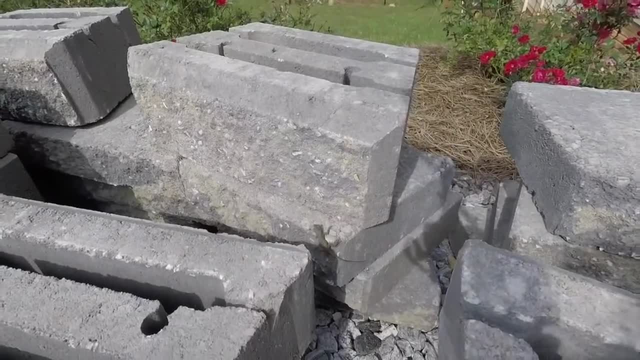 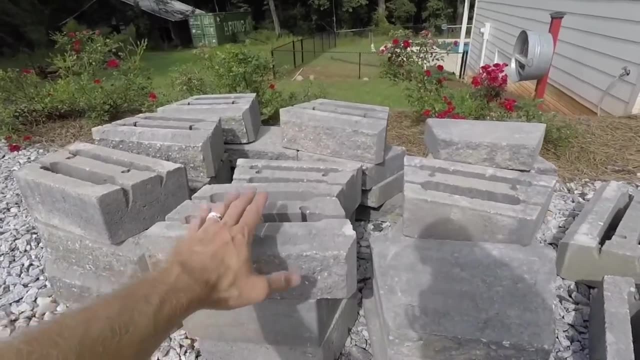 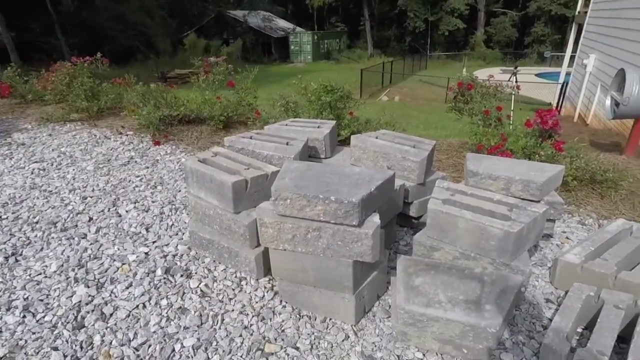 lizard right there. We have so many little lizards out here. now The step: this is a retaining wall block, and then I've got a cap block to put on top of them, and that's basically what it's going to be. 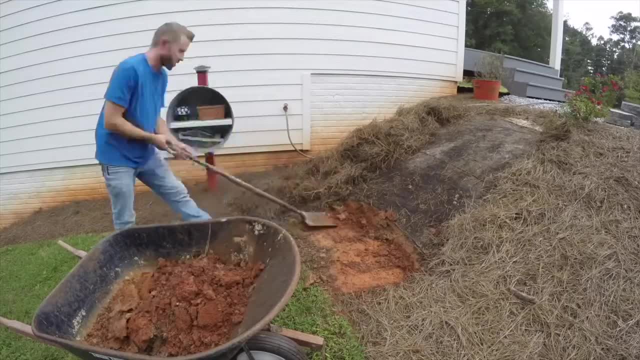 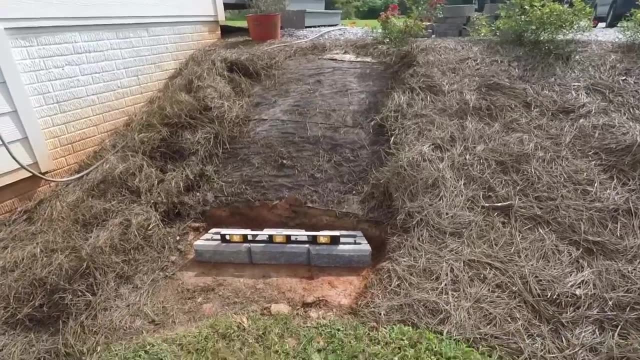 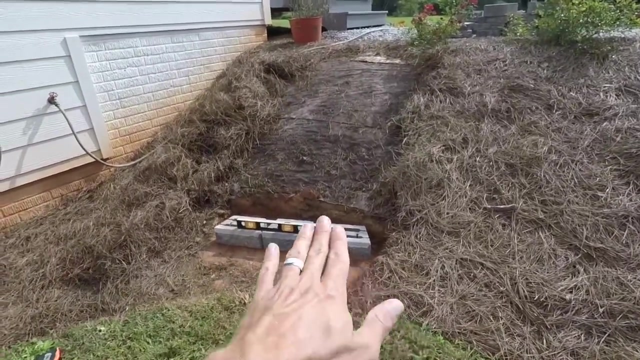 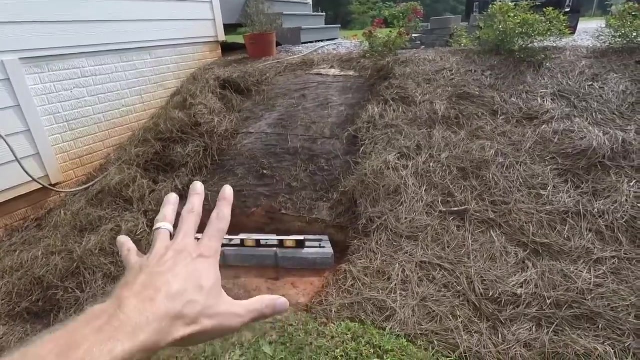 I don't really like the way this looks. I think I'm going to have to dig it out further over here because we kind of want it curved. So this is going to take a lot longer to figure out than I thought. I think once I get the first one or two steps figured out, it'll be quick. 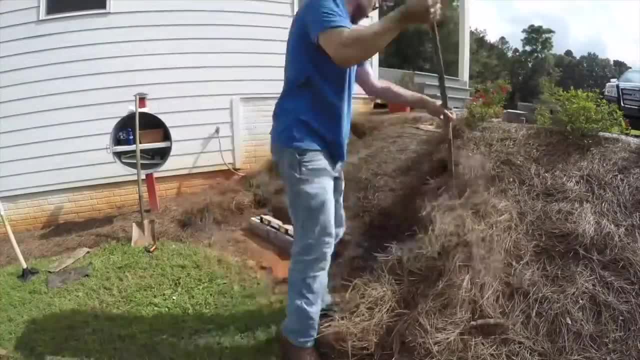 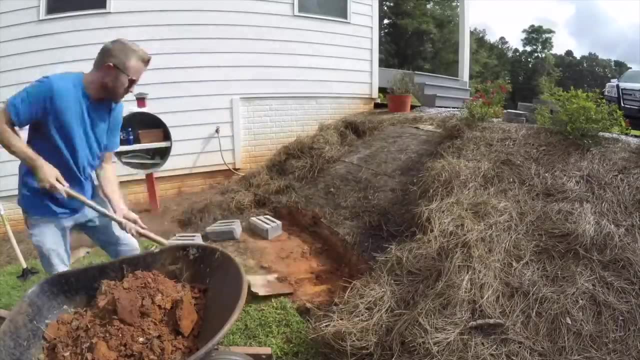 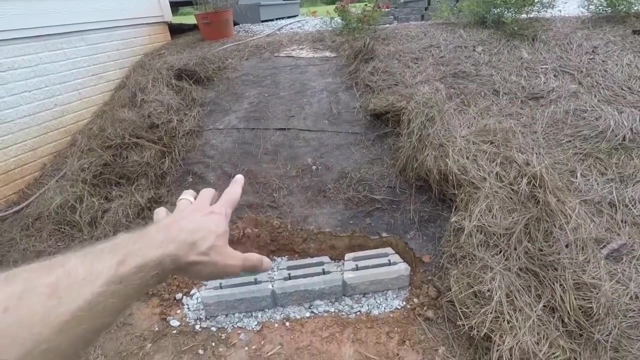 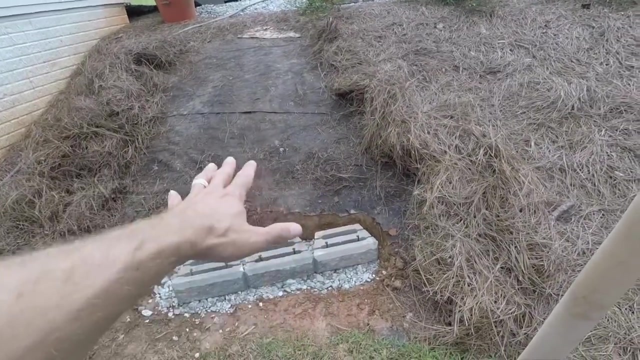 I missed B Helping me out. I am so frustrated. Last time I built these steps on another house I lived in, I did not use any gravel or any kind of sand or anything. I put three steps in. I dug the dirt out, packed it down, put the steps in. They lasted for years but I made a video about. 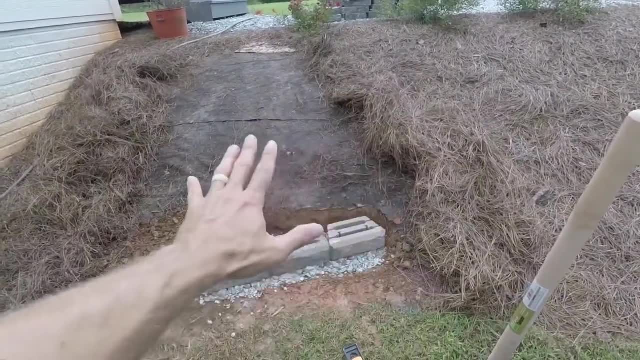 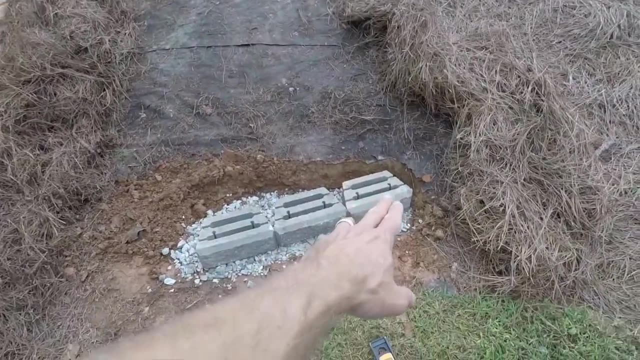 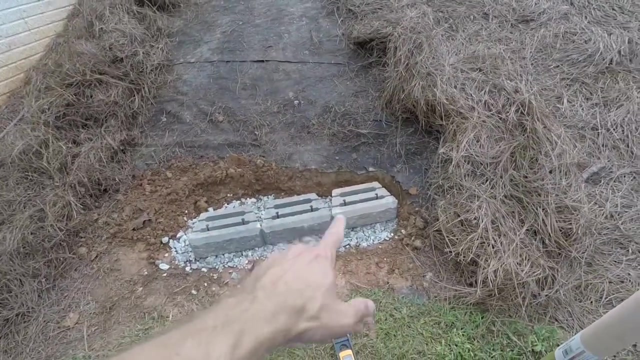 putting this driveway in here. This dirt is just. it's terrible. It does not compact very good, It just stays damp and clumpy and moist, Anyway. so I've got gravel here. I've taken some gravel from my driveway and I think we're going to try that It's already looking better. Put the gravel down. 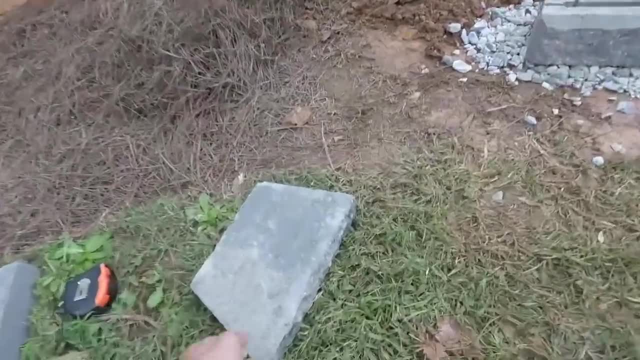 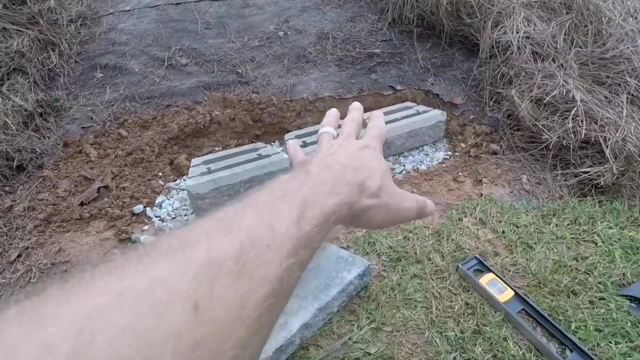 and I pack it down. Now I've got these end caps, not end caps, caps, Basically. I've got a bunch of these. I'm going to put these on top. We're going to glue them on The ones on the other side. 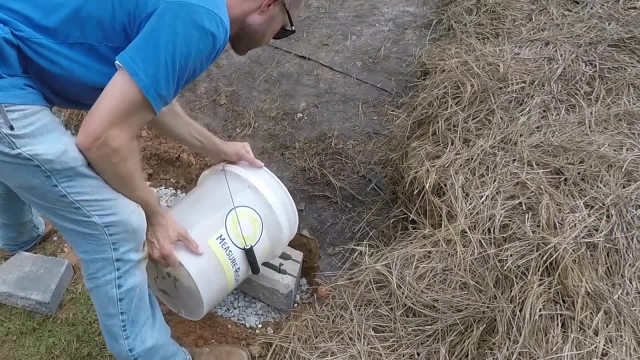 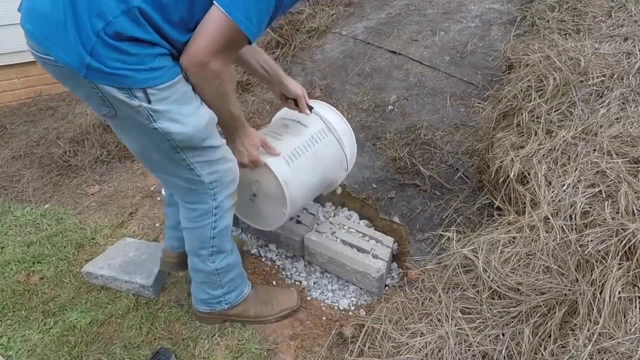 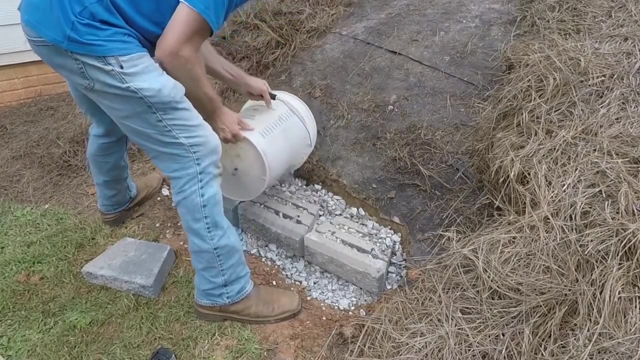 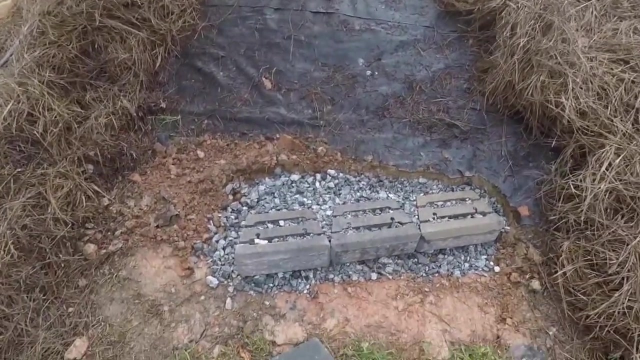 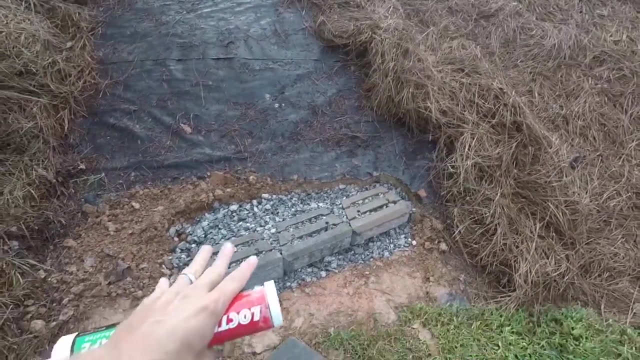 on the end I'm gonna have to cut. it's been raining. I'm not gonna get these done today, so this is what my gravel looks like. originally I had no plan to use any gravel, but it turned out good. it's gonna make a much more stable base. 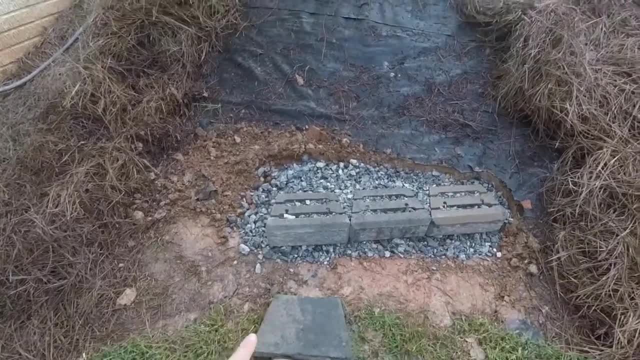 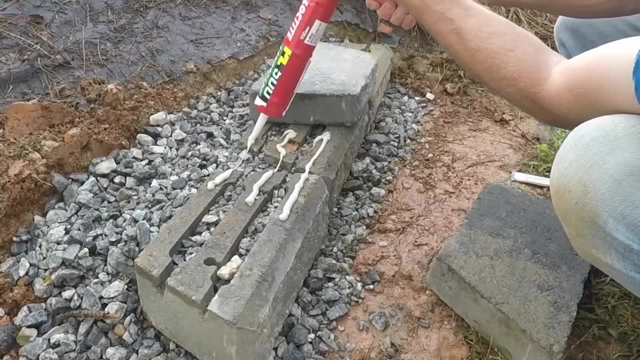 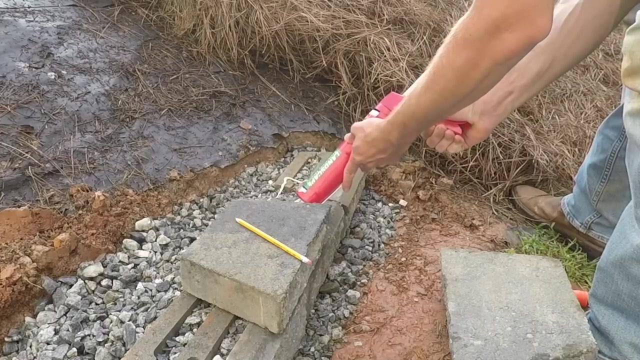 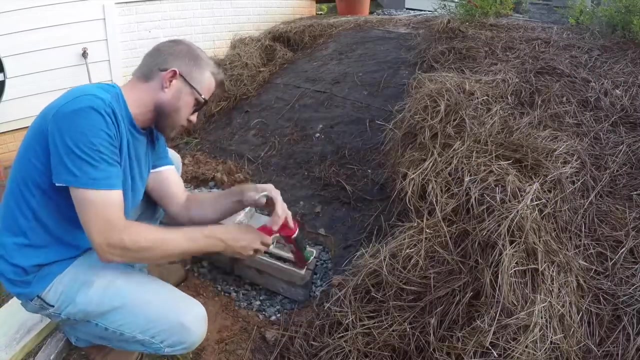 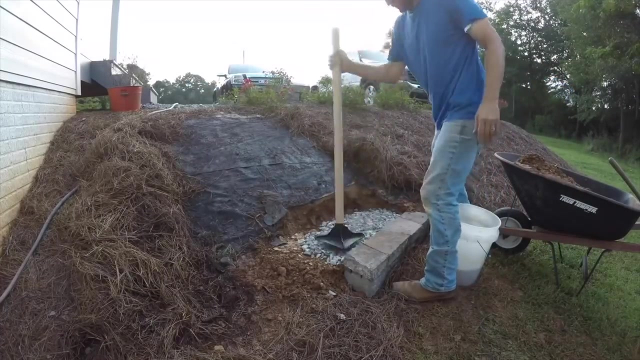 the next thing I need to do. I'm gonna glue on the the caps. I'm gonna use this landscape construction adhesive. I'm just gonna wanna put this under the edges so it doesn't paint on the outside a little bit, and I'm gonna get rid of that old paint there and I'll 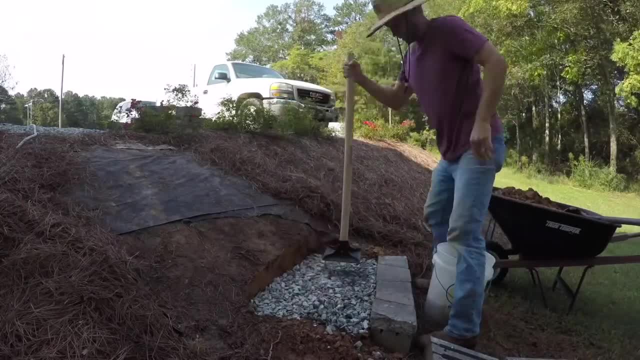 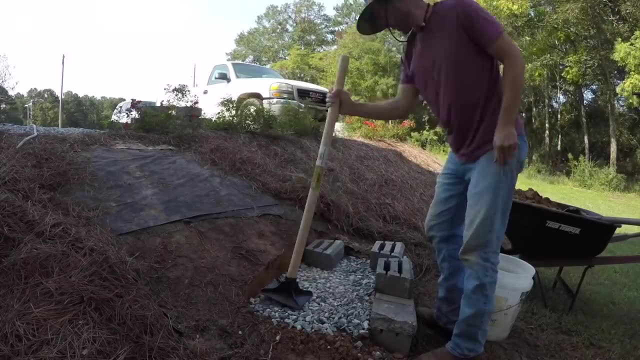 just trim that and put it on the side so I don't have to have an old paint that I'm going to use. and then I'm gonna go into one half with the new paint and I'm just gonna put it under the outside of the владi to get rid of the 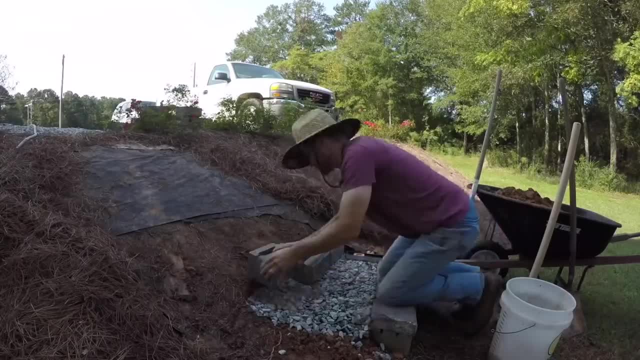 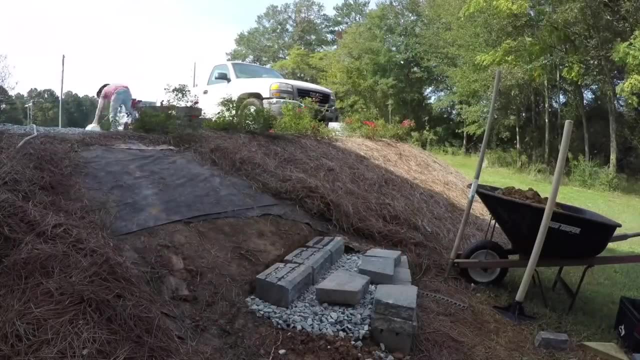 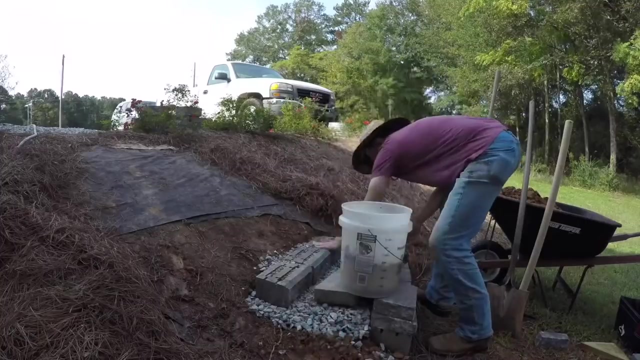 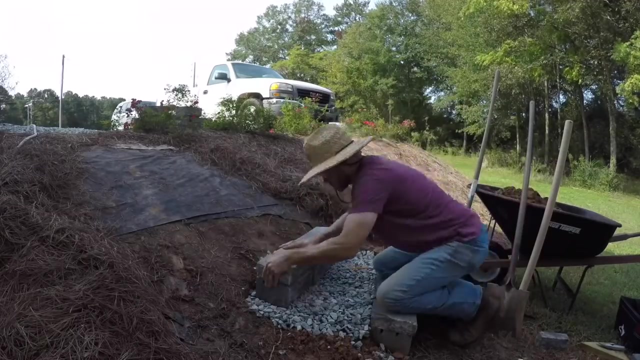 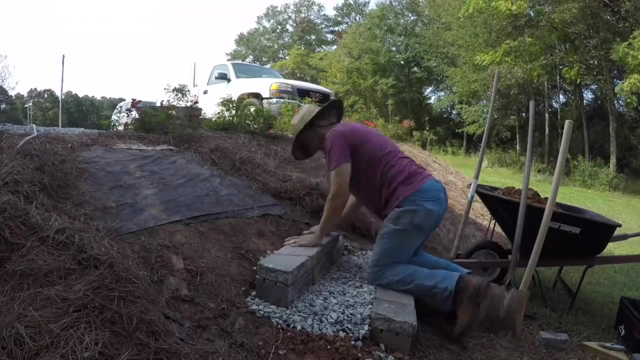 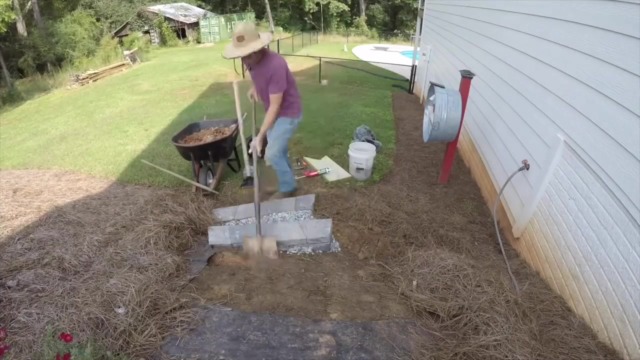 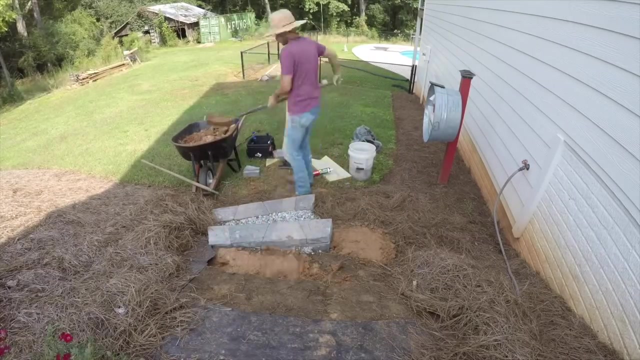 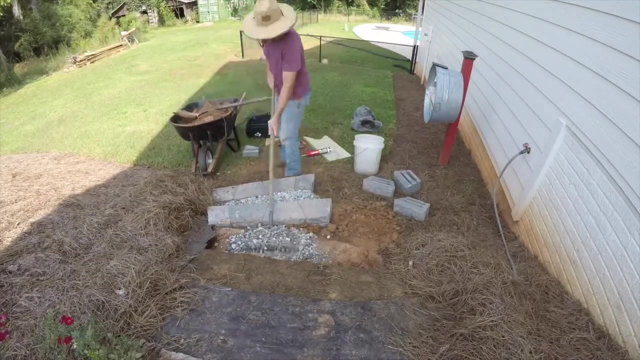 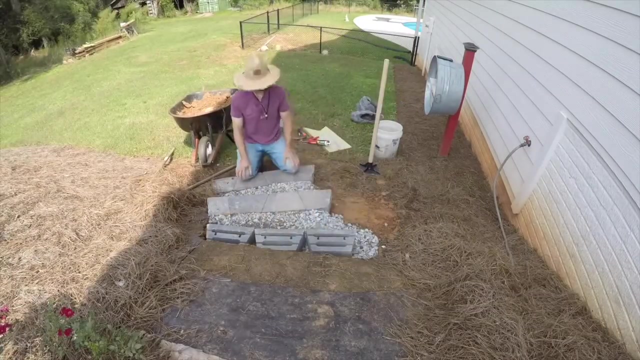 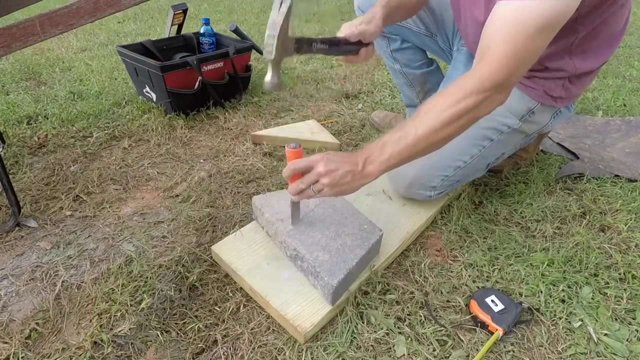 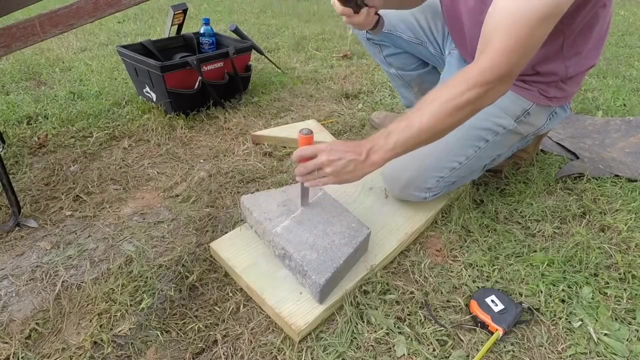 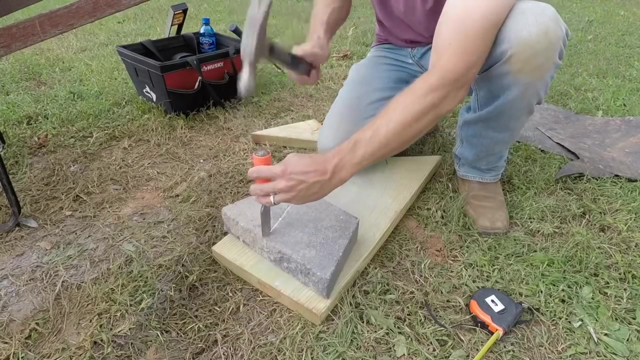 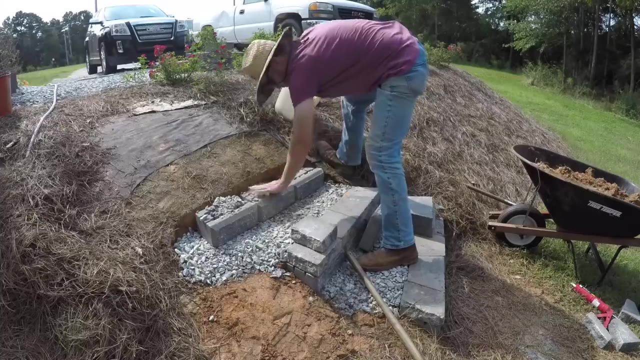 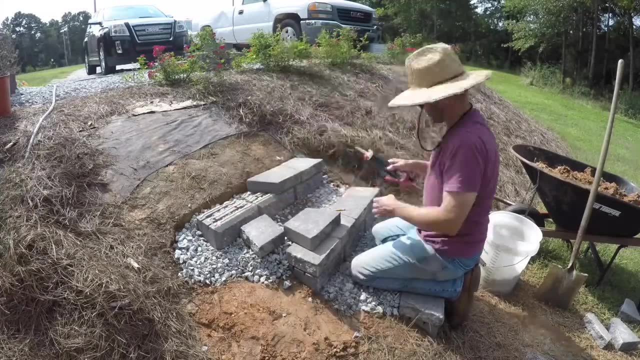 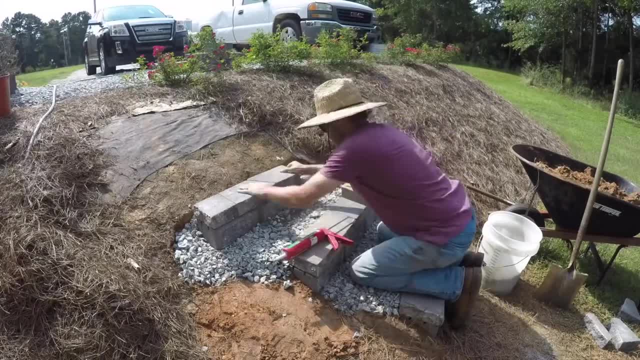 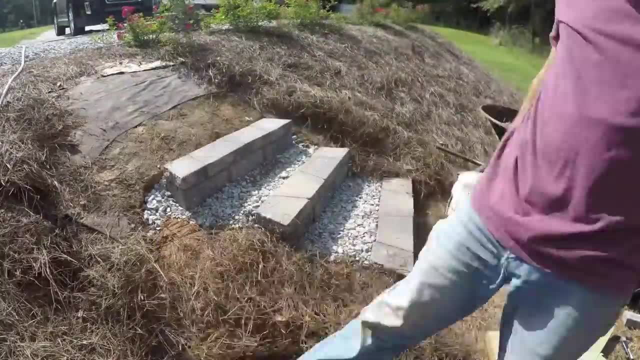 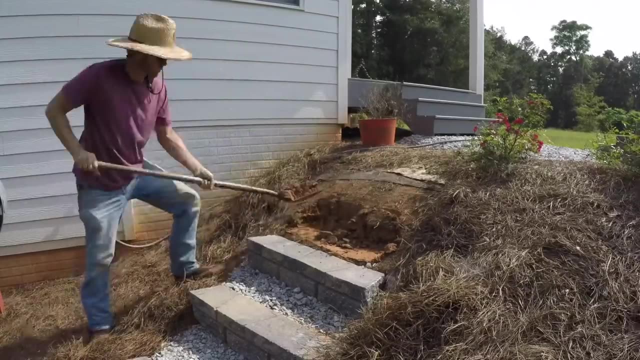 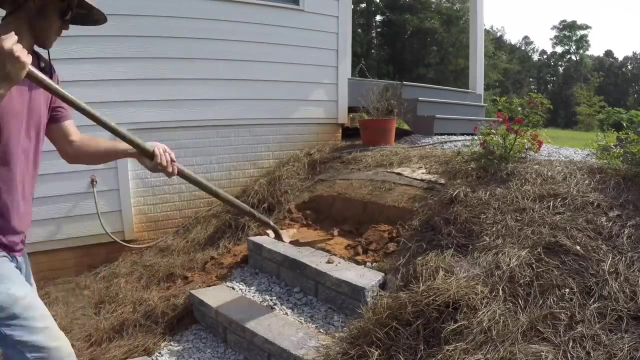 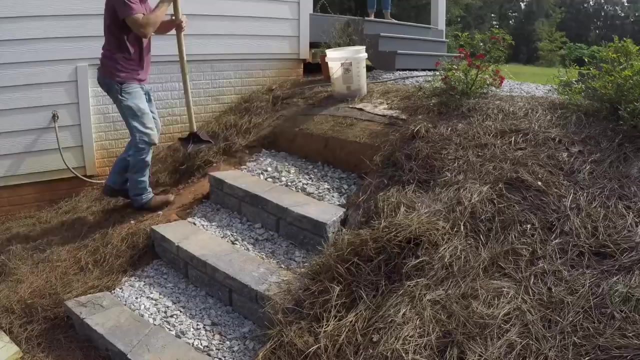 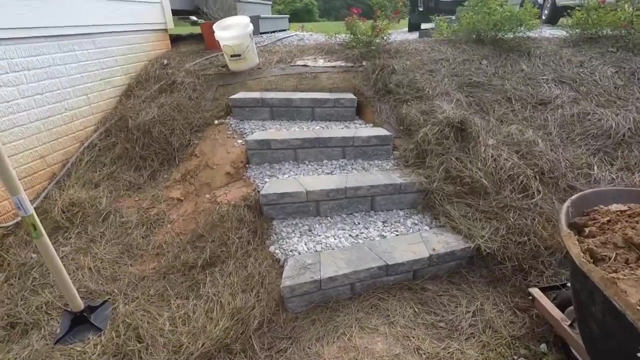 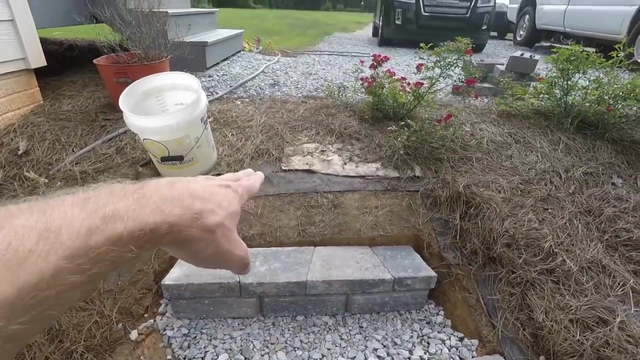 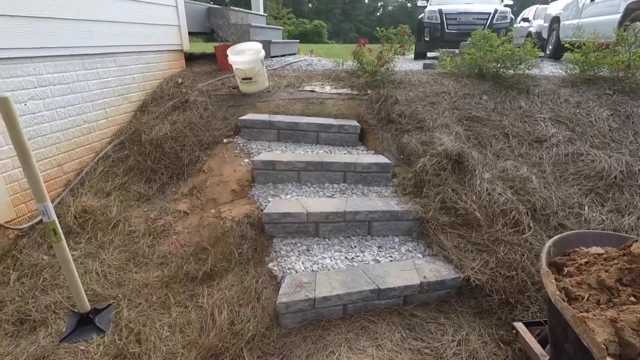 Thank you. These steps are starting to look pretty good. I still have to glue this, glue that down. dig out my last step. I'm happy that five is going to make it, so I don't have to spend any more money on these. 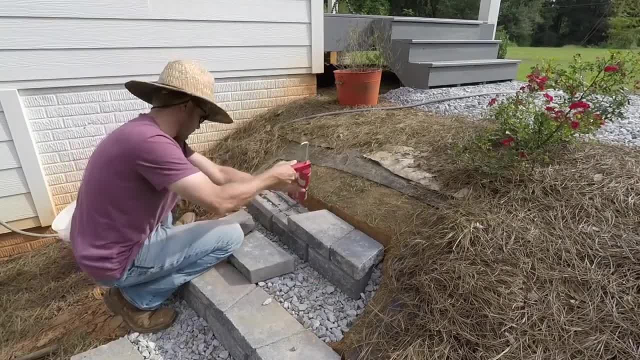 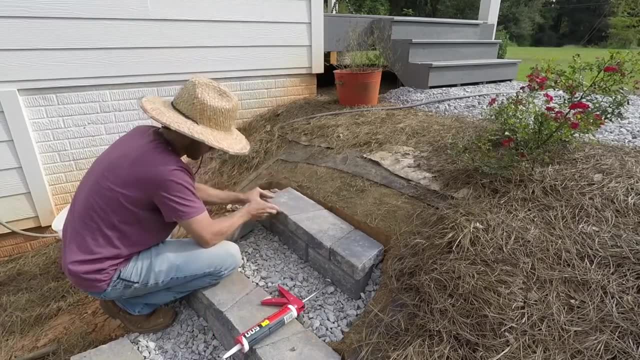 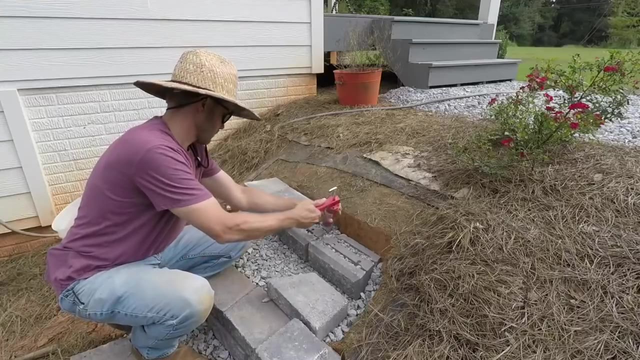 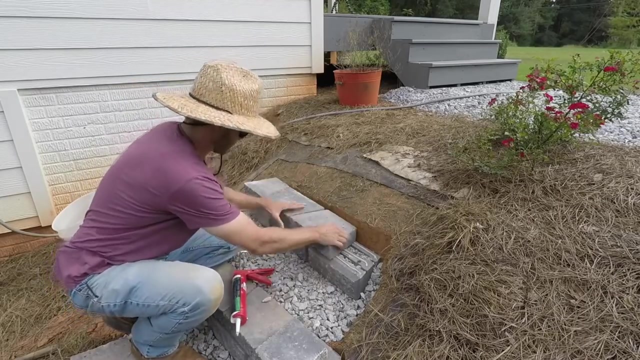 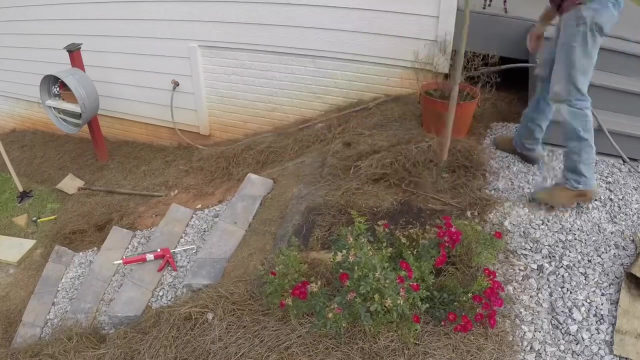 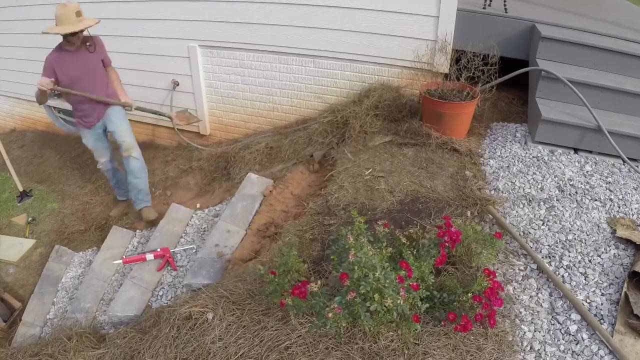 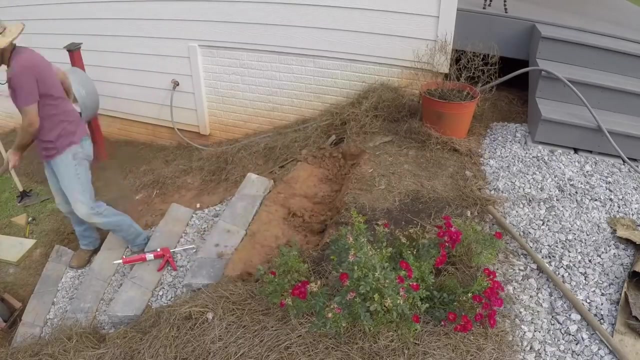 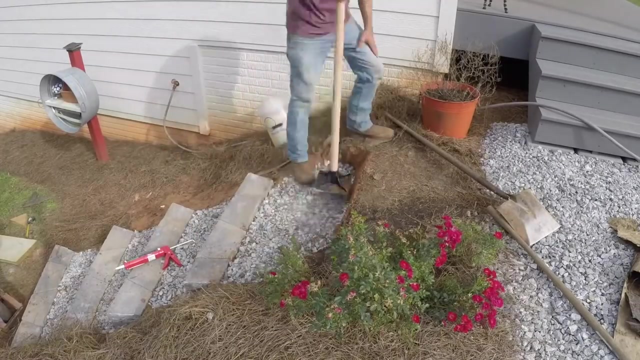 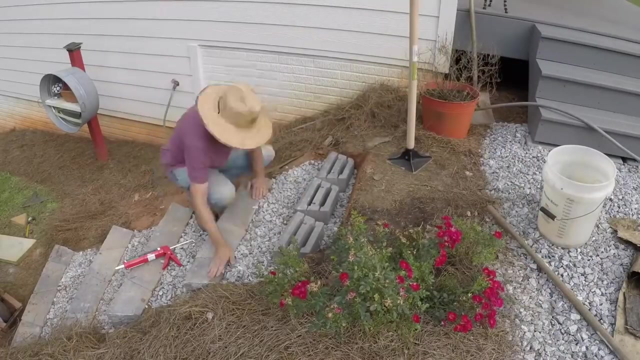 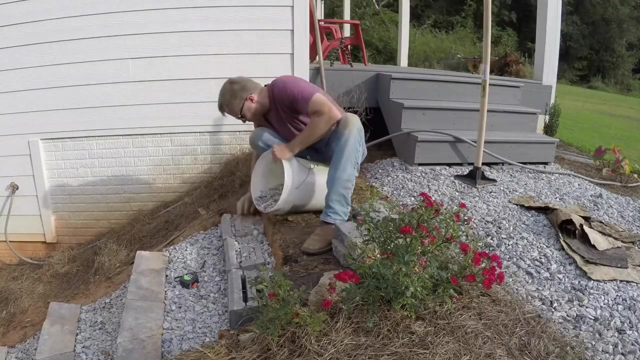 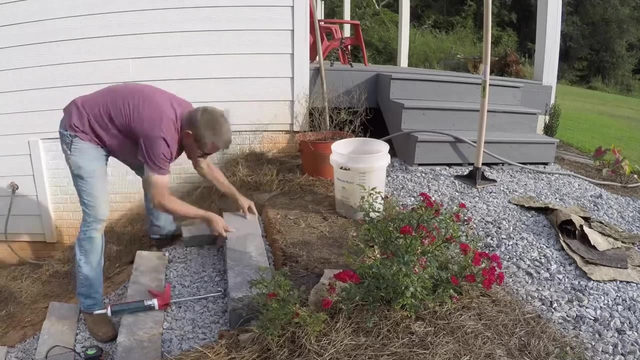 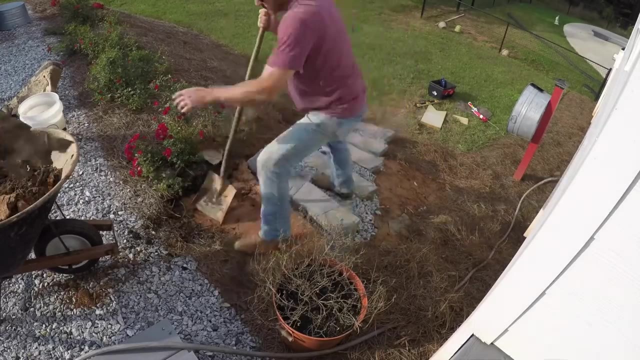 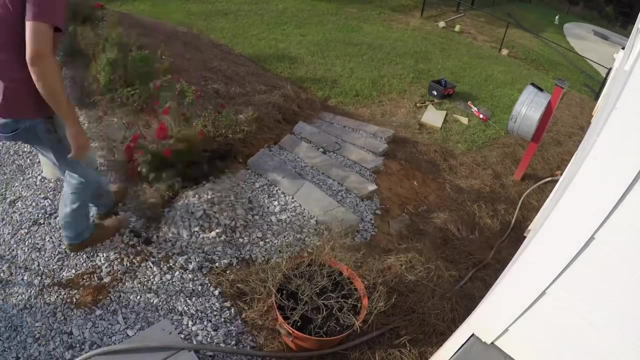 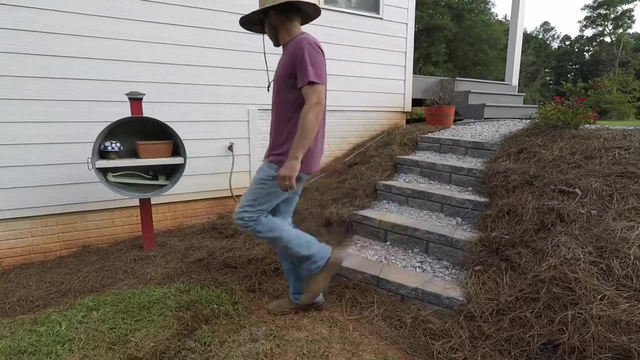 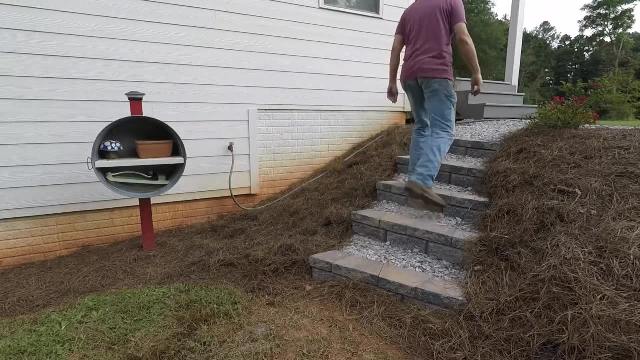 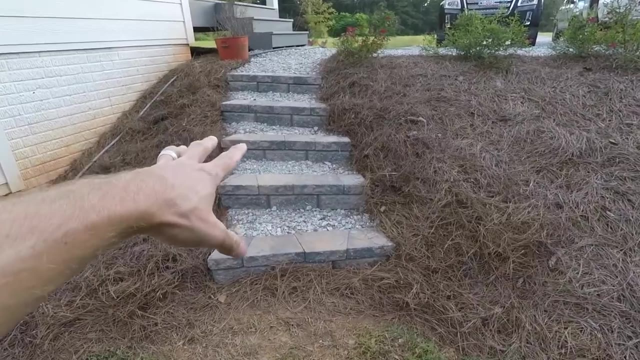 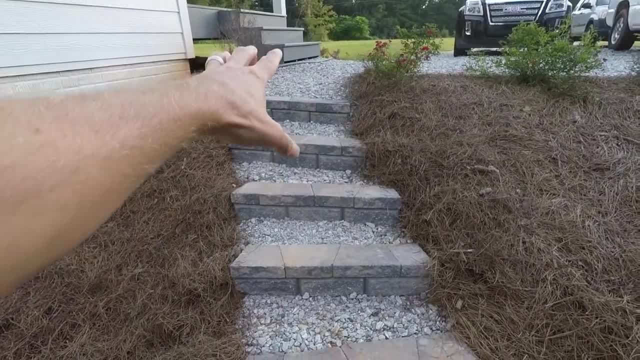 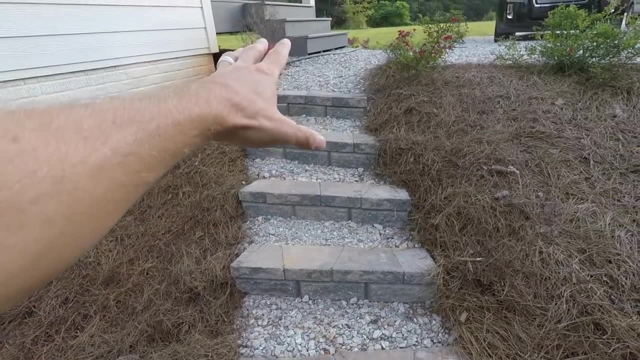 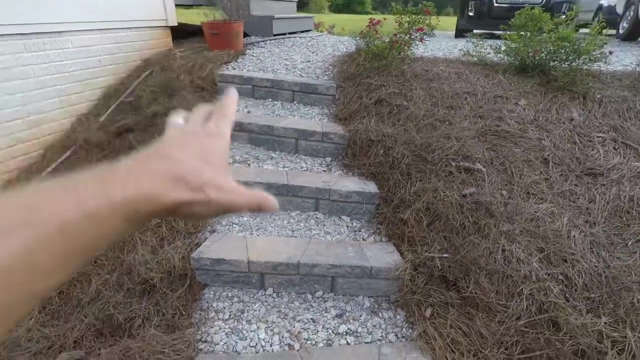 I was having to walk down them very carefully. The glue or the adhesive has not set up. I think it takes seven days. I think it said seven days for the glue. I need to cure the adhesive. Whatever, By next weekend these should be pretty solid and I can run up and down them. 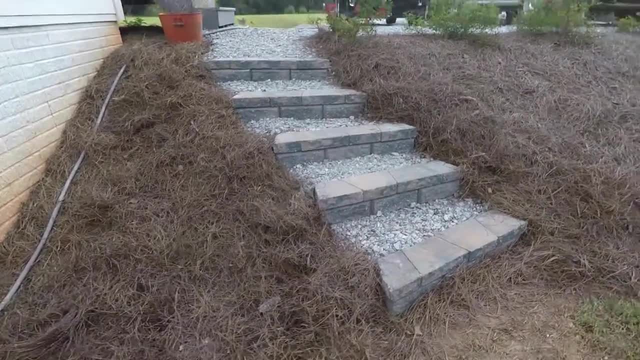 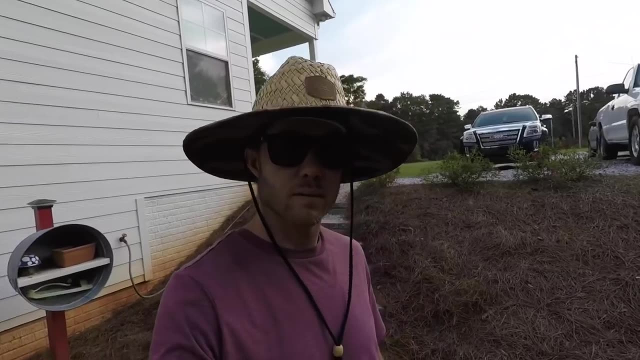 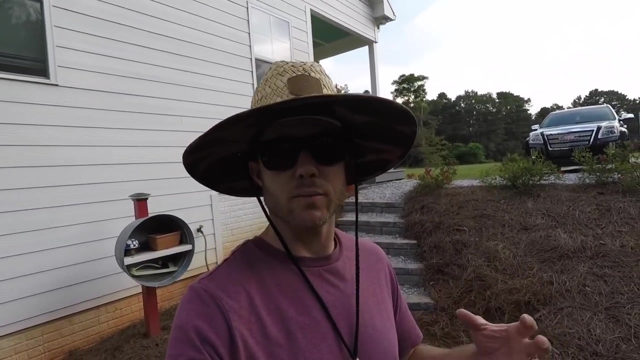 I've got about $100 in materials in this project and it took me two days to do it. I actually started last weekend and I finished today. I think these steps turned out great, Considering that I really didn't have an exact plan or an idea about what I was going to do. 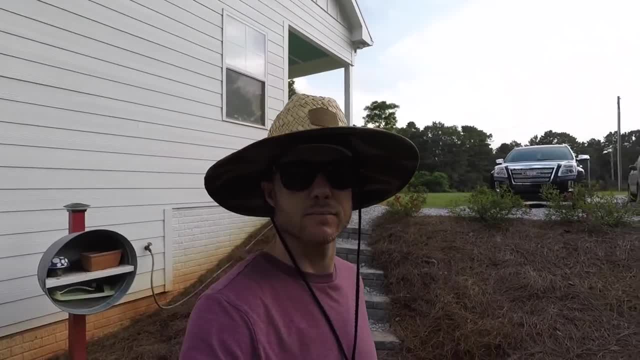 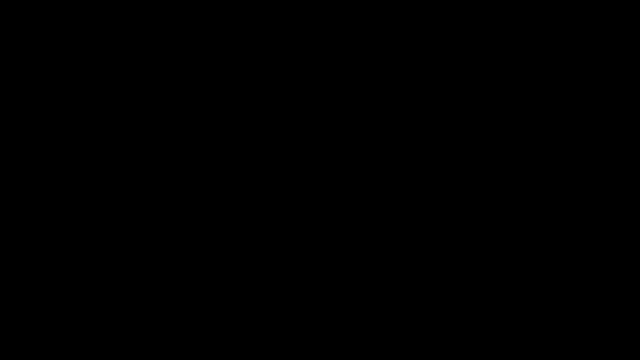 I just knew I wanted steps in this here. I'm very excited to see how this tool will help me. When I was a kid, I had no idea I was going to make a tool with this tool. The tool was the V-tip and the handle. 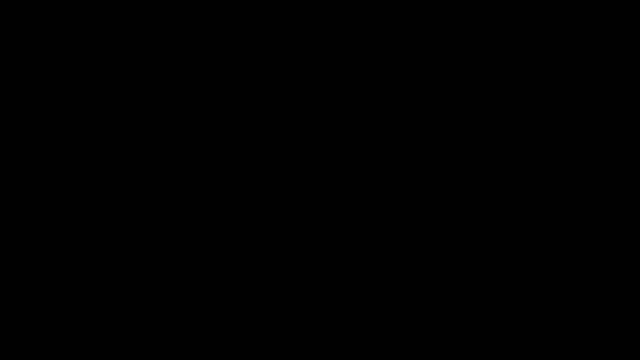 I discovered that the needle was made from the thread. It's like a traditional charm that has been around since Andalusian people. It's a really good tool. It's one of the best tools I've ever had. I just wanted to test it. I wanted to see how I would apply it to my actual work. I just wanted to check how it would work. I used it on the back, So then I can't just tell it.